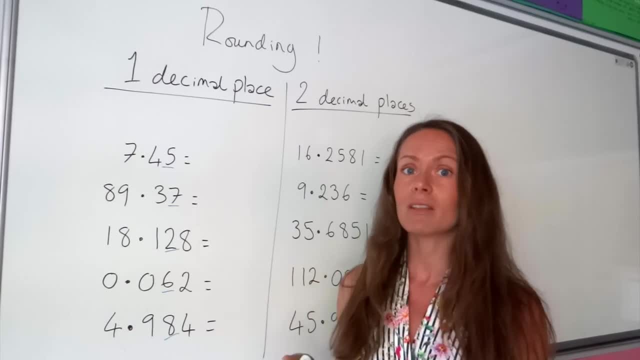 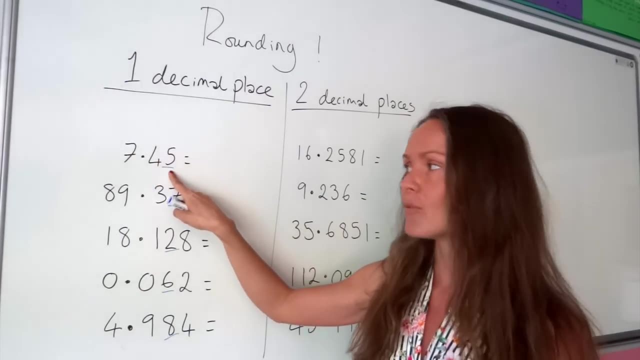 number is five or bigger than the number five, And if it's smaller than five then we don't round up. So in the first one I can see that the second number after the decimal point is the number five. So it means it rounds this number up one, So it changes to a five. 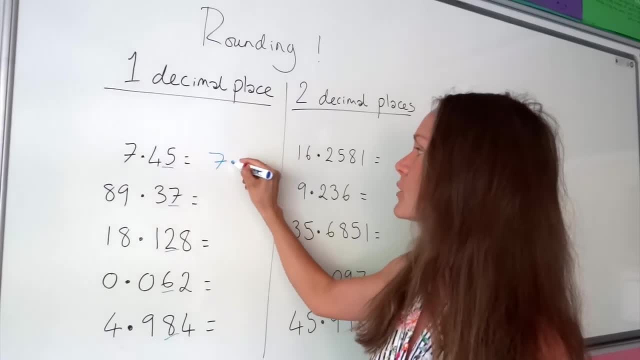 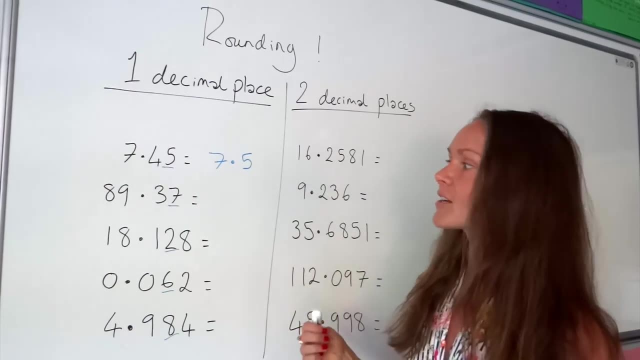 So we're left with 7.5.. So that's the first one And I can see that's one decimal place, because I've only got one number after the decimal place. All right, let's look at the next one. So again, the second number after the decimal. again it's bigger than five, So it means you. 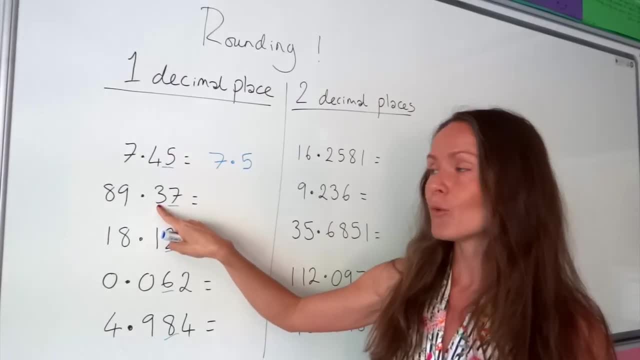 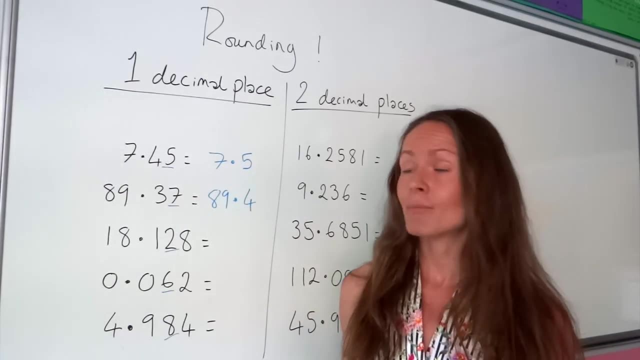 round up. So this number changes to the number four. So we're left with 89.4.. On to the next one. So this time the number that's two after the decimal point is the number five. So we're left with: 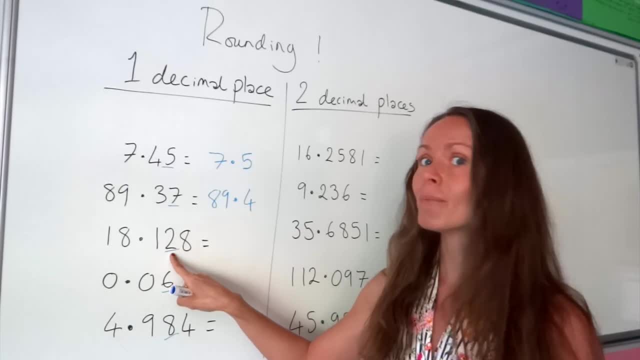 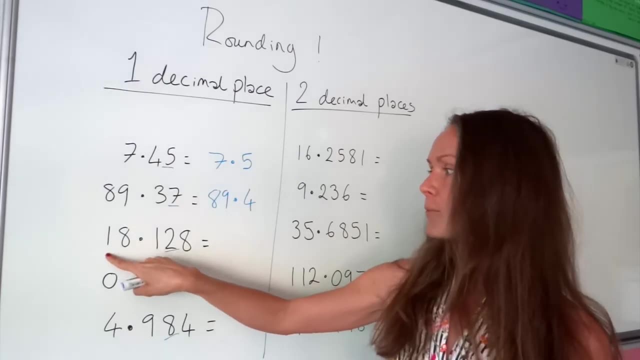 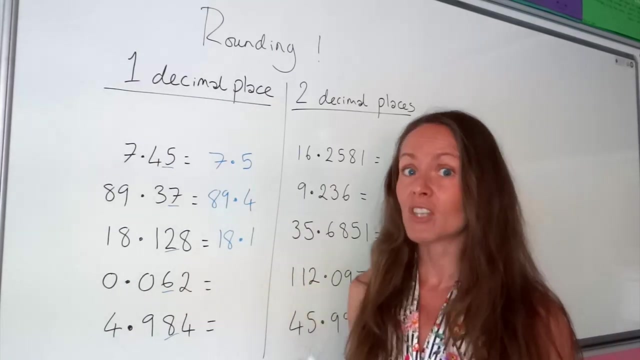 a decimal. here It's smaller than five. So remember, when it's smaller than five we don't round up. So this time this number, here it stays the same. So we're just left with 18.1.. OK, now on to this one down here. Remember we're checking the second number after the decimal. 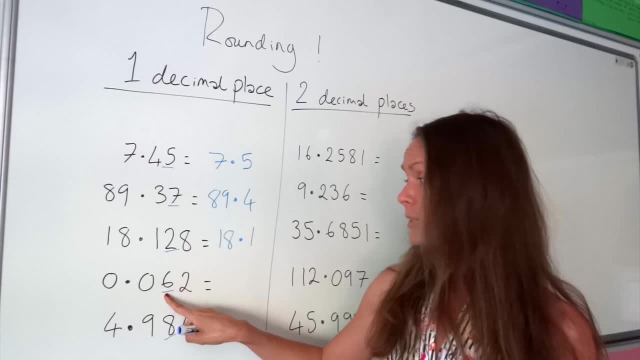 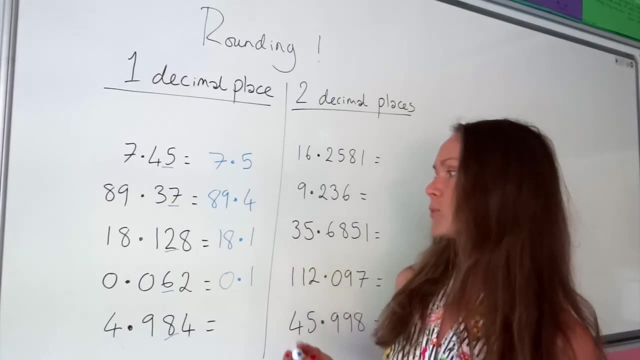 place And it's bigger than five, which means we round this number up one, So it changes to 0.1.. On to the last one. Now, this is the tricky one, So make sure you're listening. So again. 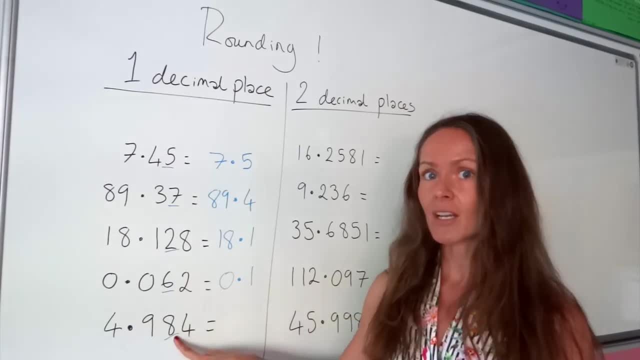 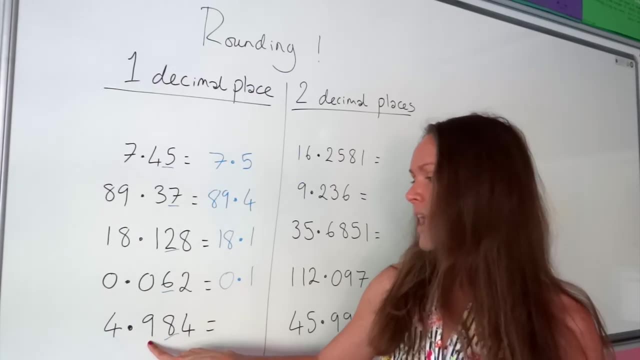 we check the second number after the decimal, It's bigger than the number five, which means we have to round up. So when we round this number up we get the number 10.. Except, we can't squeeze in the number 10 here. We have to spread it out. So what happens to that number 10? is that nine? 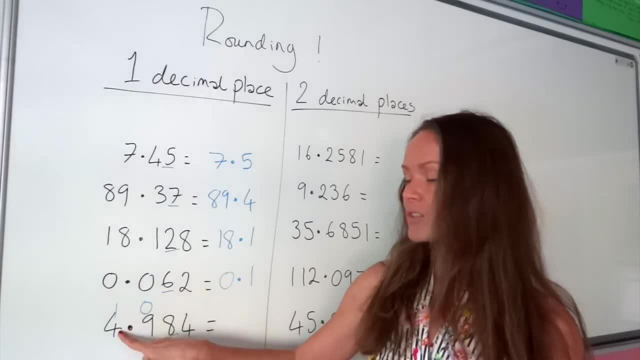 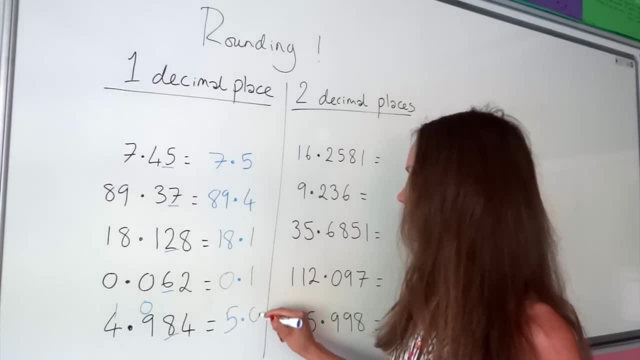 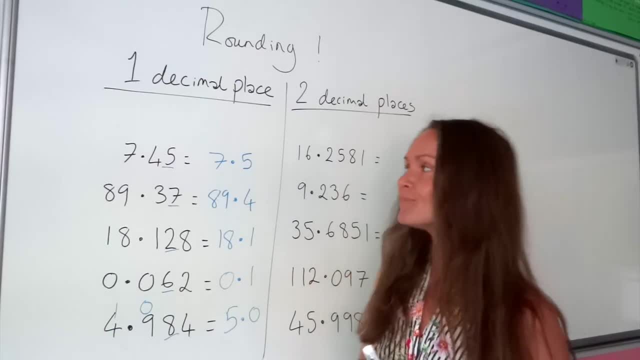 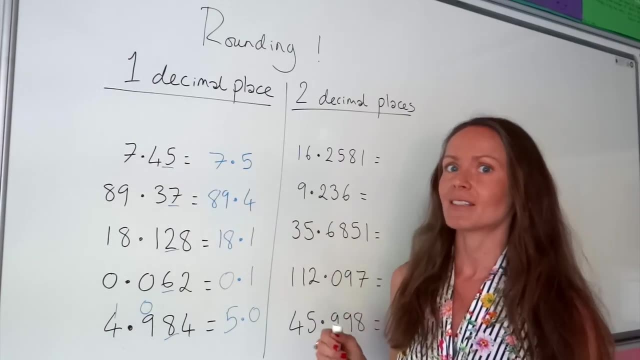 because I'm going to do some more examples like that one later on. okay, Now, this time, if we're rounding to two decimal places, we don't check the second digit after the decimal anymore, We check the third one. So this time we're looking at this number here. 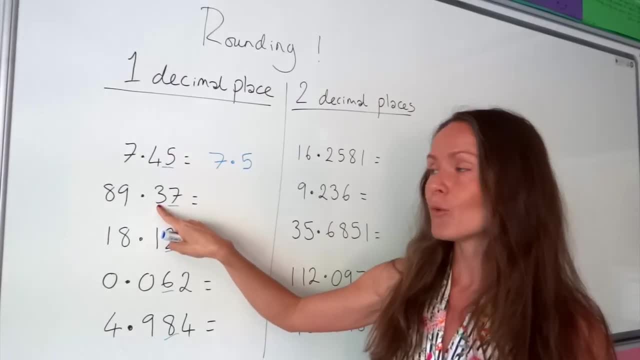 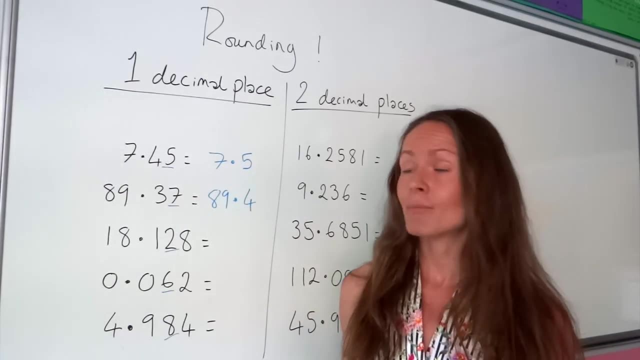 round up. So this number changes to the number four. So we're left with 89.4.. On to the next one. So this time the number that's two after the decimal point is the number five. So we're left with: 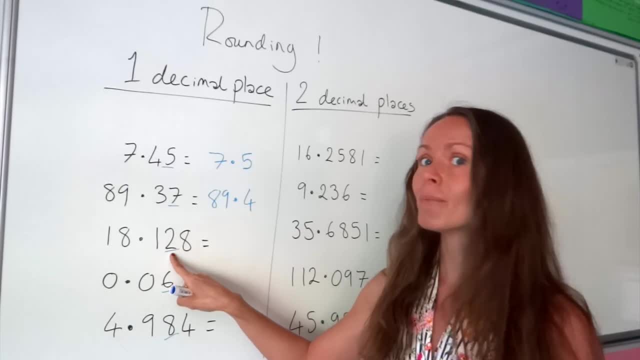 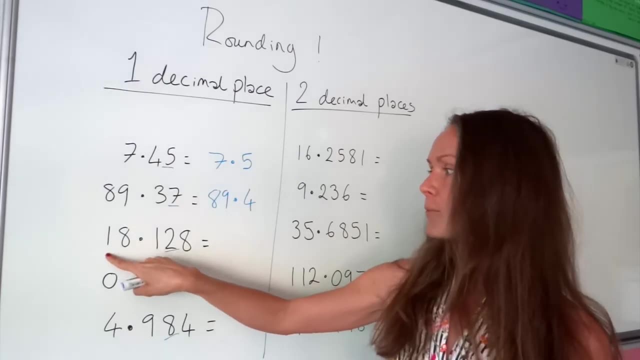 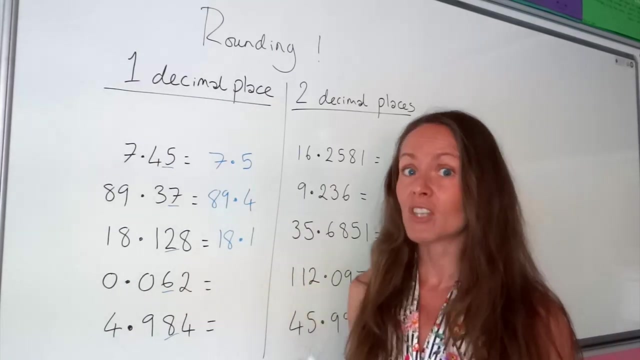 a decimal. here It's smaller than five. So remember, when it's smaller than five we don't round up. So this time this number, here it stays the same. So we're just left with 18.1.. Okay, now on to this one down here. Remember we're checking the second number after the decimal. 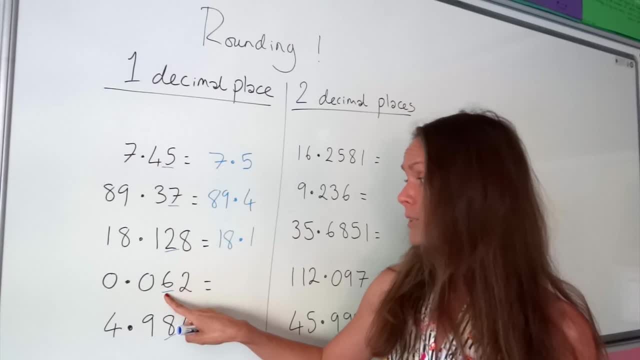 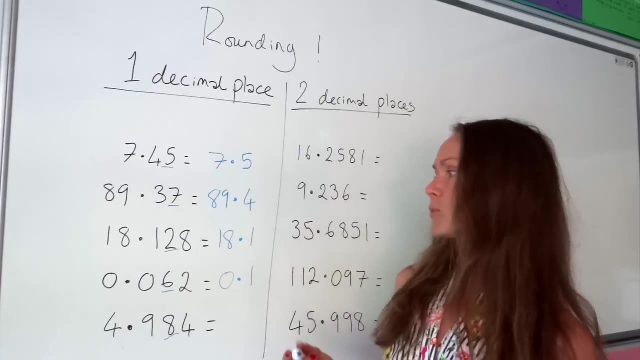 place And it's bigger than five, which means we round this number up one, So it changes to 0.1.. Now on to the last one. Now, this is the tricky one, So make sure you're listening. So again. 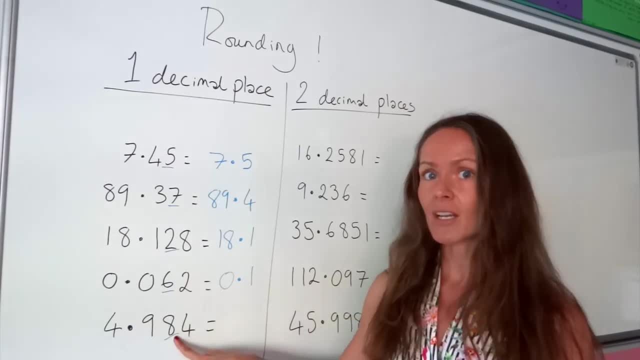 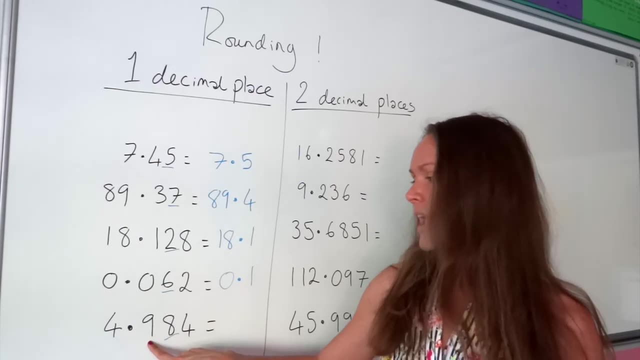 we check the second number after the decimal, It's bigger than the number five, which means we have to round up. So when we round this number up we get the number 10.. Except, we can't squeeze in the number 10 here. we have to spread it out. So what happens to that number 10? is that nine? 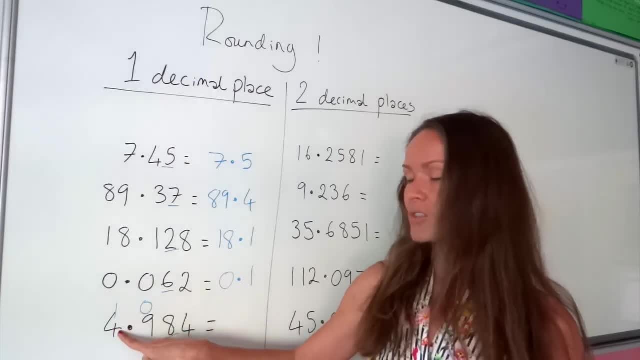 changes to a zero, And that one is added to the number here, So it changes to a five, So we're actually left with 5.0.. Now don't worry if you didn't quite get that one, because I'm going to do some more examples like that one later on. okay, 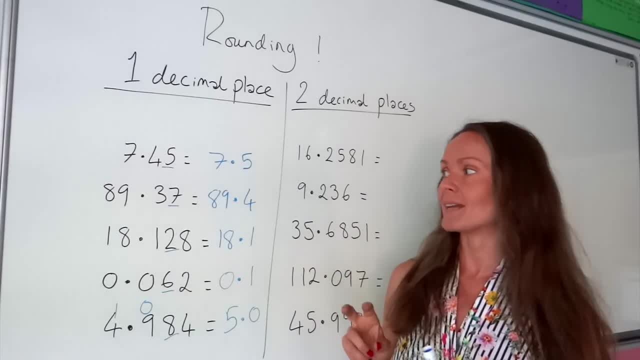 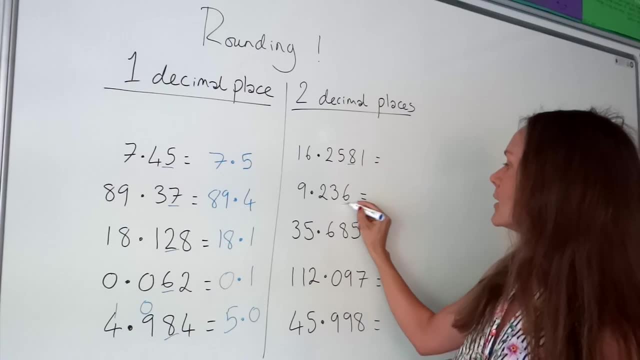 Now, this time if we're rounding to two decimal places, we don't check the second digit after the decimal anymore, We check the third one. So this time we're looking at this number here to see if it rounds the one next to it up or not. 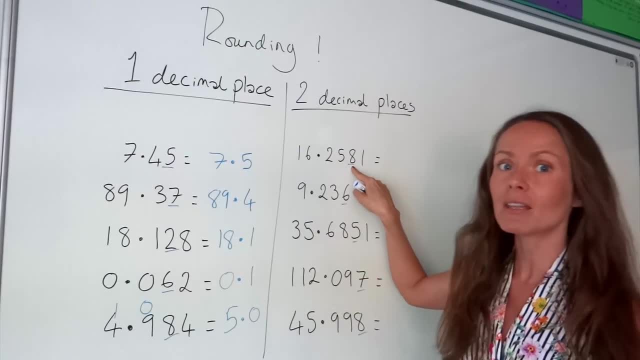 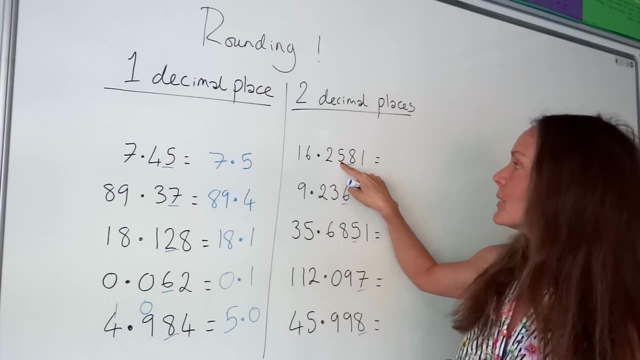 So in this one here the third number is bigger than 5.. Remember that means we round up. So this number here changes to the number 6.. So we're left with 16.26.. So everything else stays the same. 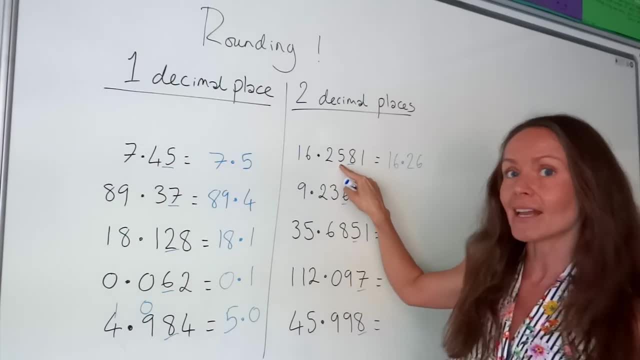 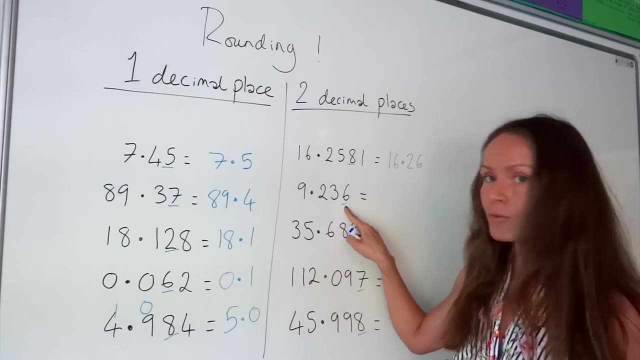 It's just this one, directly next to the number 8, that gets rounded. Okay, this one here. Again, the third number after the decimal point is bigger than 5, which means it rounds this number up. Remember, Remember, these stay the same. 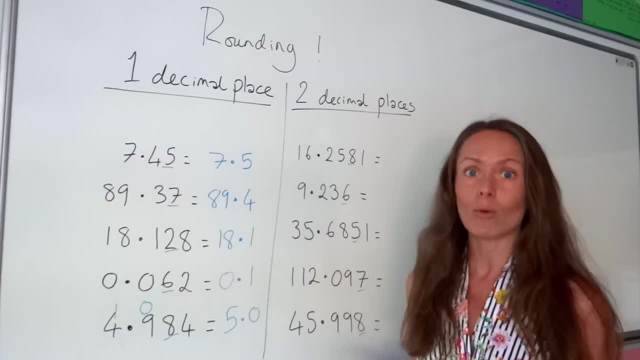 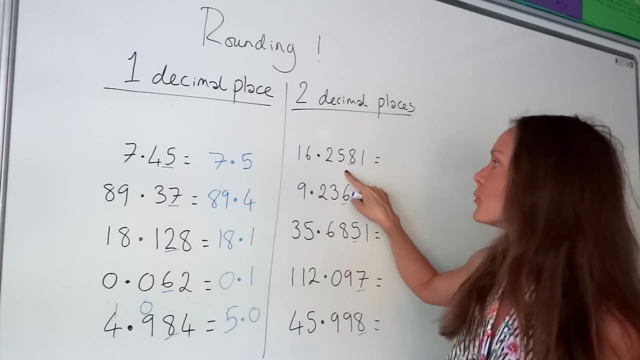 to see if it rounds the one next to it up or not. So in this one here the third number is bigger than 5. Remember that means we round up. So this number here changes to the number 6.. So we're left with 16.26.. 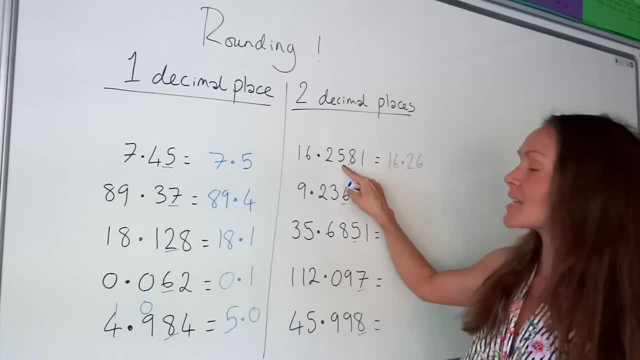 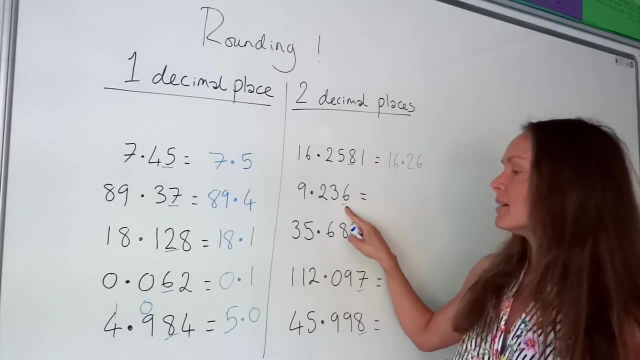 So everything else stays the same. It's just this one, directly next to the number 8, that gets rounded. Okay, this one here Again. the third number after the decimal point is bigger than 5, which means it rounds this number up. 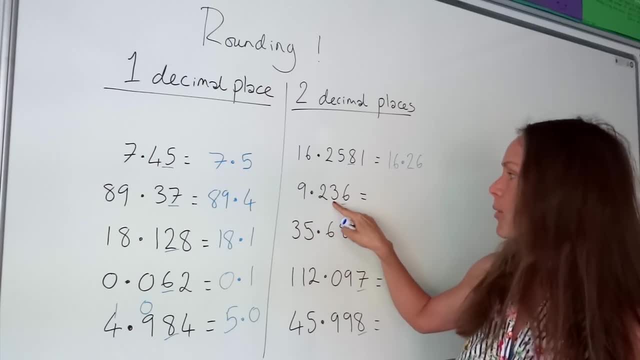 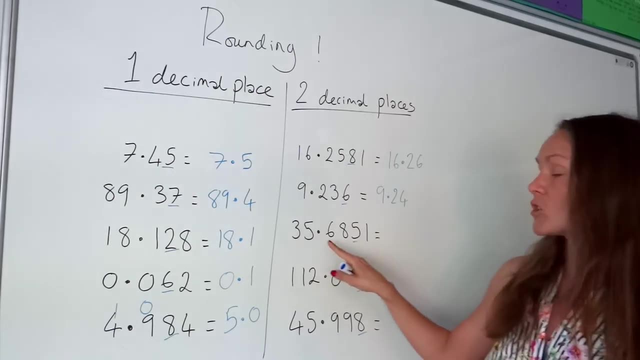 Remember, Remember, these stay the same. It's only this one that moves up one, So we're left with 9.24.. All right, now this one down here Again, we're checking the third number after the decimal point. 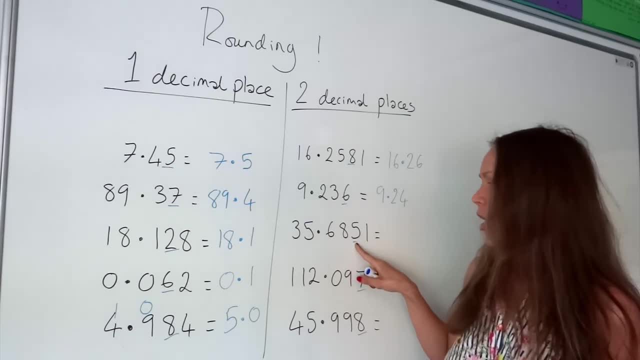 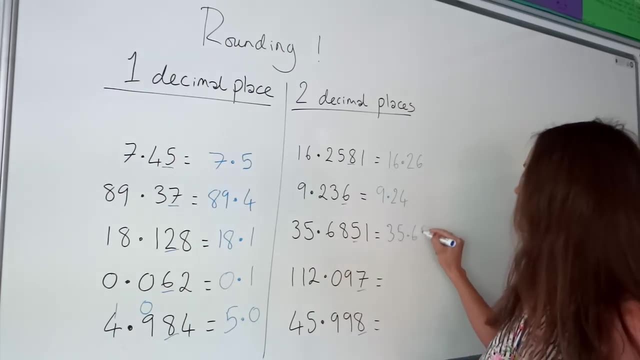 So this time it's the number 5, which means we have to round up. So this number gets rounded up to the number 9.. So we've got 35.69.. Okay now. so these are the hard ones that are very similar to this one I did over here. 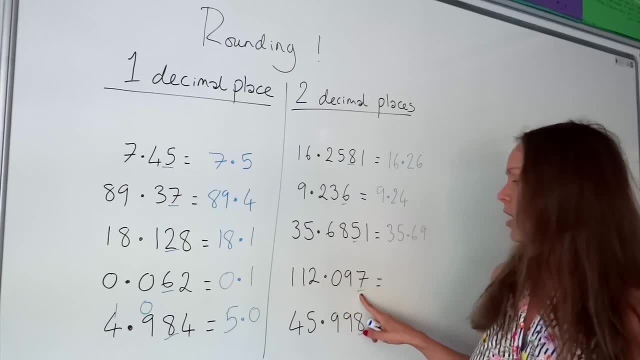 So this time, when I check the third one again, it rounds up. So this number gets rounded up one, But the number that comes after the number 9 is the number 10.. So remember, this is when it has a knock-on effect. 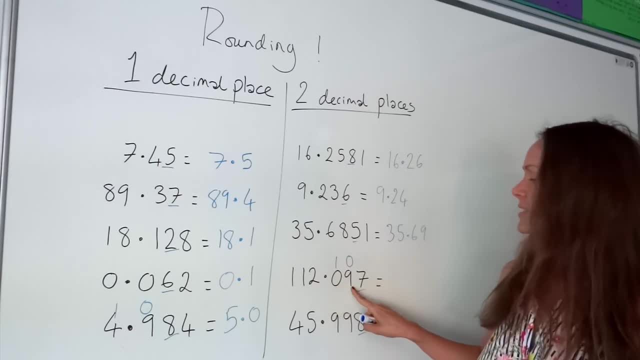 on the number in front as well. So this number changes to a 0, and the number 1 in number 10 changes this one up one, So it gets added to the number 0. So we're left with 112.10.. 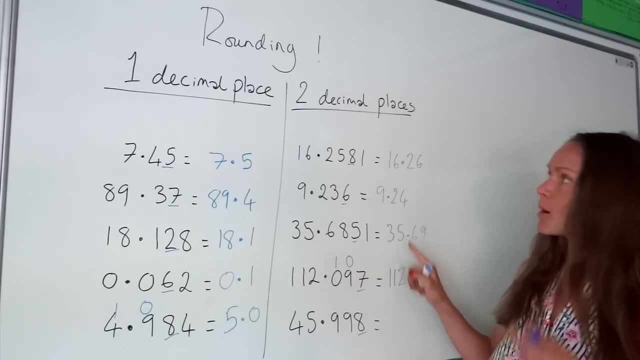 And you have to write that 0 at the end because, remember, we're rounding to two decimal places, which means you need to have two numbers after the decimal point. So if you only wrote that, which is the same thing, that would only be one decimal place. 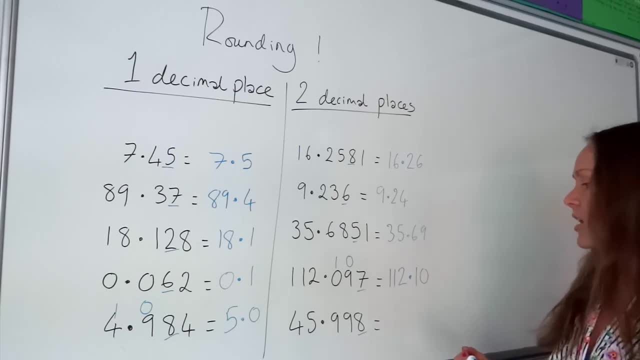 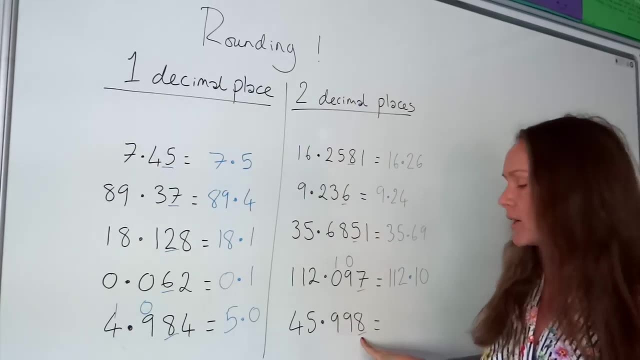 You need to leave that in as well. Okay, and the last one. Again, remember, when you're rounding to two decimal places, you check the third digit after the decimal point to see if it rounds up. And because this number is bigger than 5,. 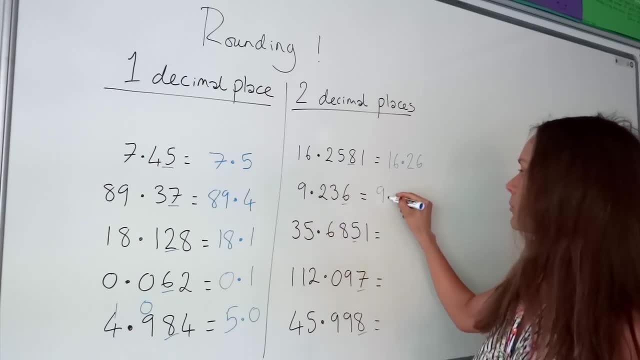 It's only this one that moves up one, So we're left with 9.24.. Alright, now this one down. here. Again, we're checking the third number after the decimal point, So this time it's the number 5,, which means we have to round up. 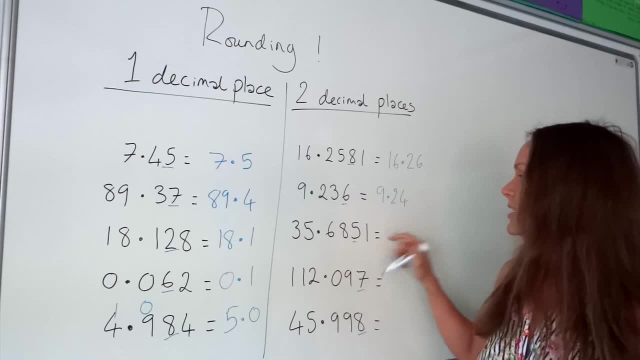 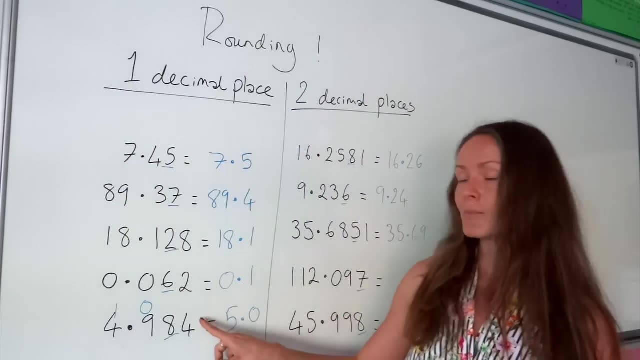 So this number gets rounded up to the number 9.. So we've got 35.69.. Okay now. so these are the hard ones that are very similar to this one I did over here. So this time when I check the third one again, it rounds up. 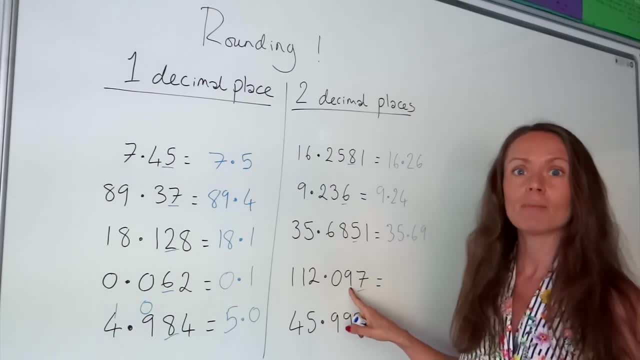 So this number gets rounded up one, But the number that comes after the number 9 is the number 10.. So remember, this is when it has a knock-on effect on the number in front as well, So this number changes to a 0.. 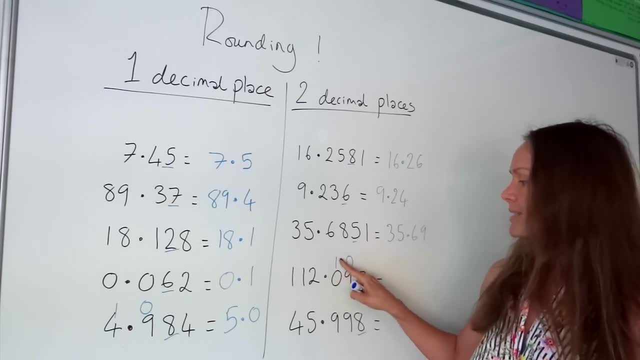 And the number 1 in number 10 changes this one up one, So it gets added to the number 0.. So we're left with 112.10.. And you have to write that 0 at the end because, remember, we're rounding to two decimal places. 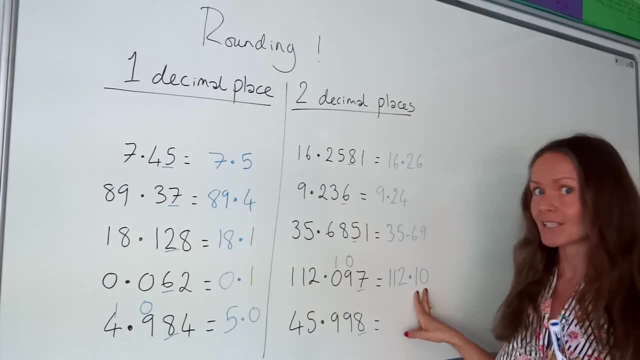 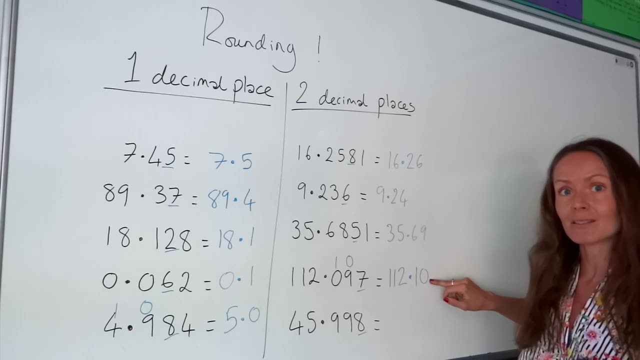 which means you need to have two numbers after the decimal point. So if you only wrote that, which is the same thing, that would only be one decimal place. You need to leave that in as well. Okay, and the last one. 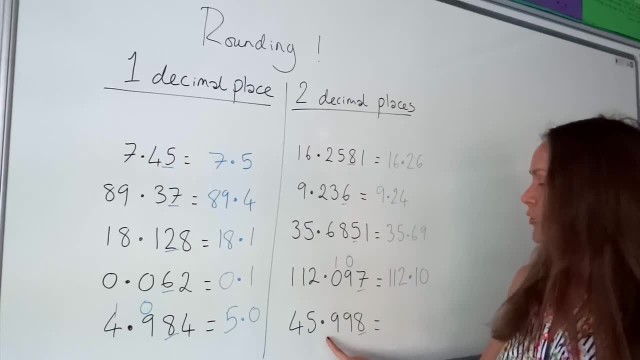 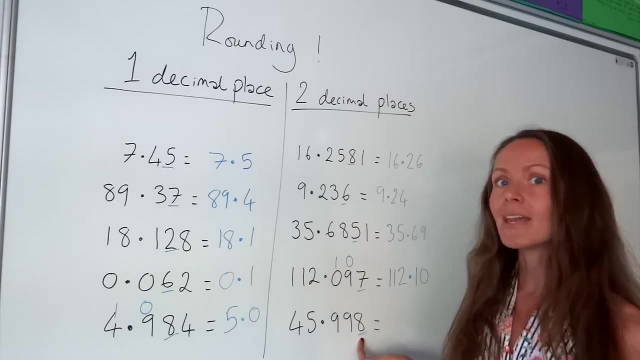 Again, remember, when you're rounding to two decimal places, you check the third digit after the decimal point to see if it rounds up. And because this number is bigger than 5, it means we have to round up And the number 9 here gets rounded to the number 10.. 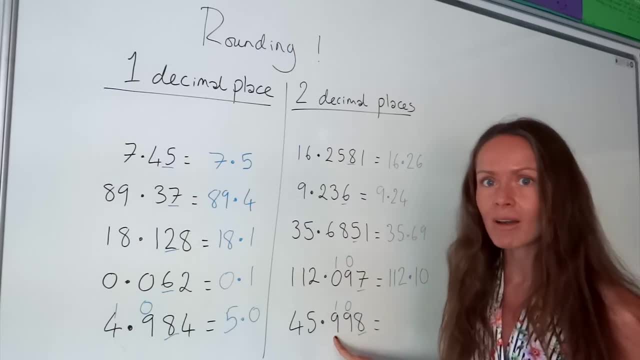 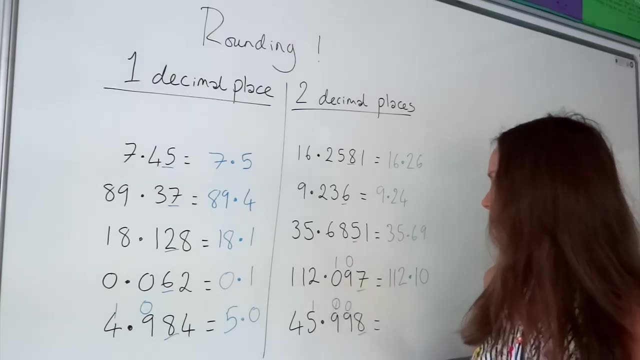 But there's a problem Because this one is also a number 9.. So this one gets rounded to a number 10 as well. So what happens is this number 1 gets added to the 5 here, So we get 46.00. 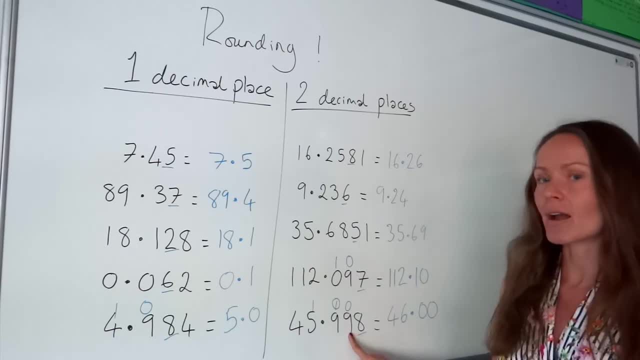 So I'll just repeat The 8. The 8 rounds this 9 up to 10, which in turn rounds that one up to 10,, which changes this one to a 6,, which makes sense because, you can see, these numbers are all bigger than 5.. 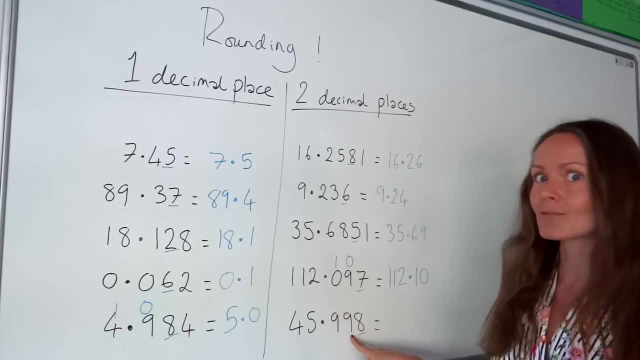 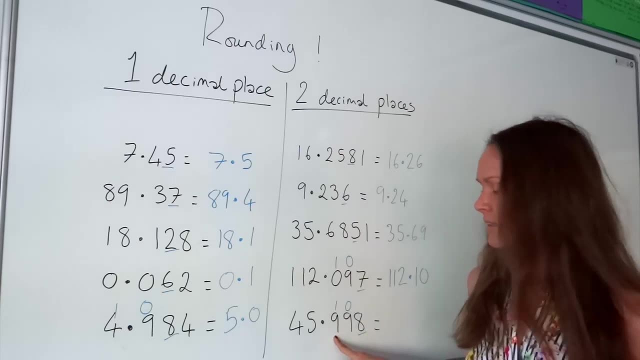 it means we have to round up, And the number 9 here gets rounded to the number 10.. But there's a problem, Because this one is also a number 9, so this one gets rounded to a number 10 as well. 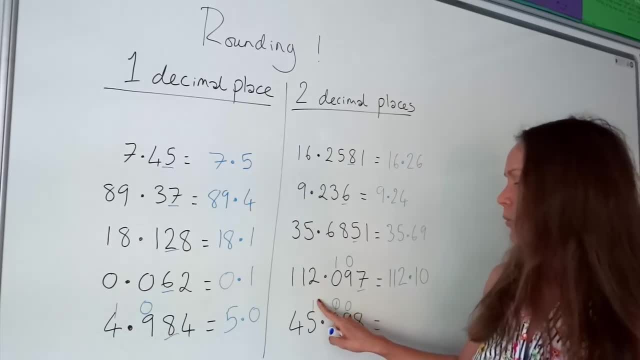 So what happens is this: number 1 gets added to the 5 here, so we get 46.00.. So I'll just repeat: It rounds this 9 up to 10, which in turn rounds that one up to 10,. 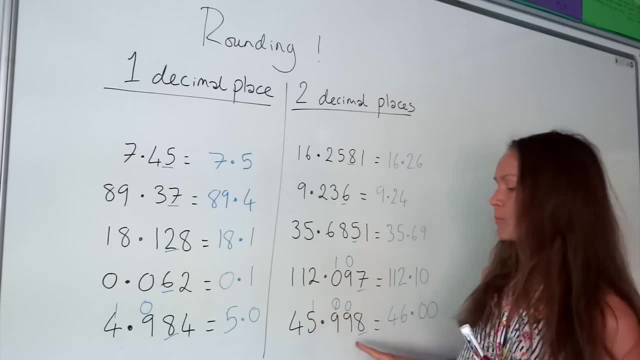 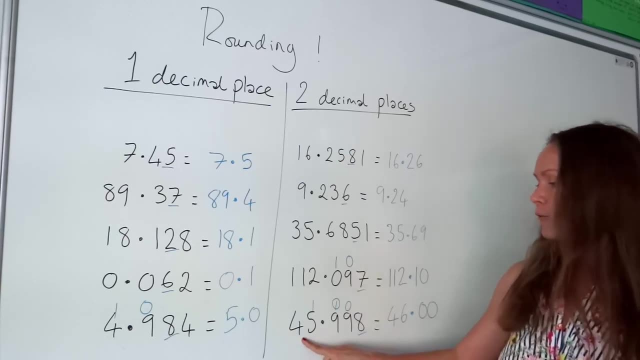 which changes this one to a 6,, which makes sense because you can see these numbers are all bigger than 5.. We should be rounding up. So the only way we're rounding up is if that 45 changes to a 46. And remember it's two decimal places. 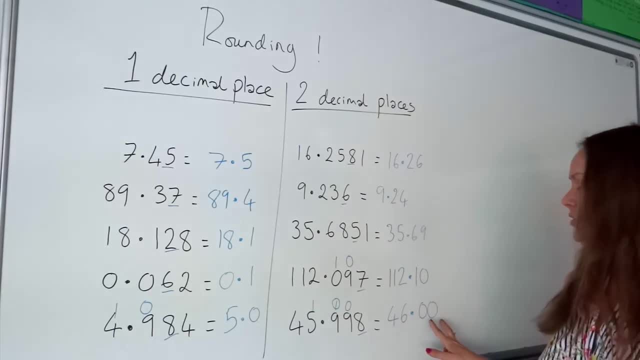 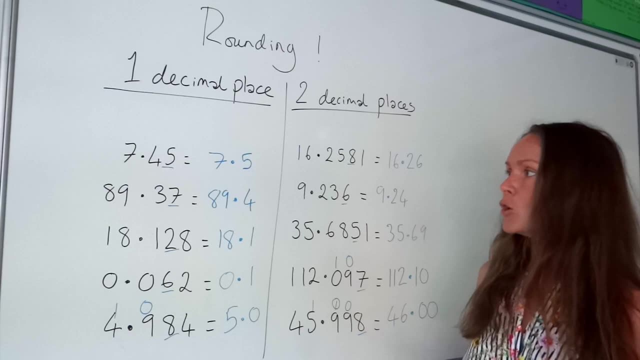 so we have to put those zeros after the decimal point so that we've got two numbers after the decimal point. So So, as you can see, that last one's quite tricky, okay, Normally when you're rounding, it only affects the number directly next to it. 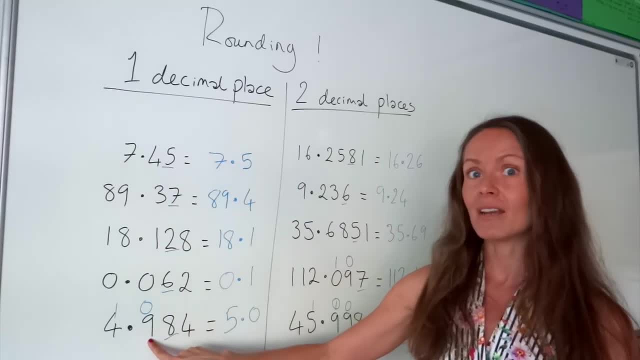 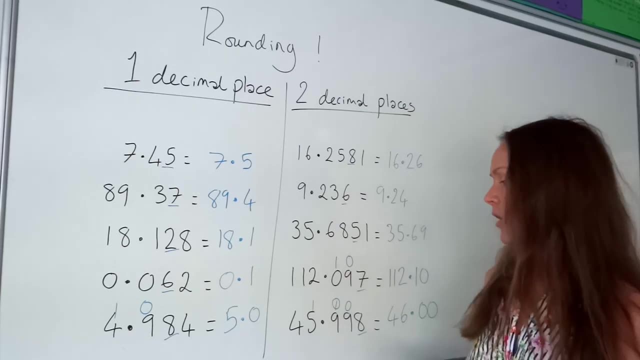 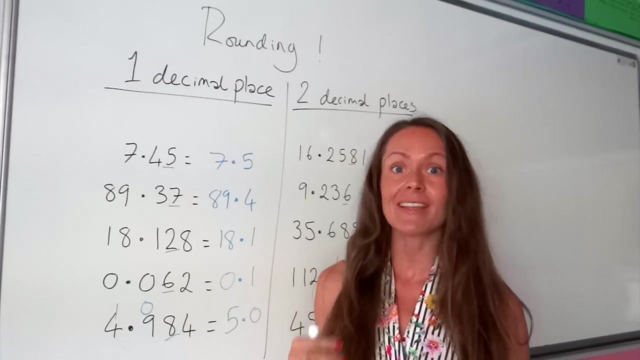 But when you're rounding and that number happens to be a number 9,, that's when it has a knock-on effect with the number that comes after that. okay, So watch out when you're rounding those number 9s. So if you find yourself rounding to three decimal places, 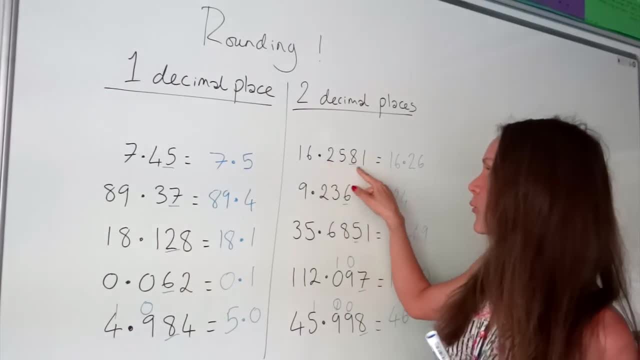 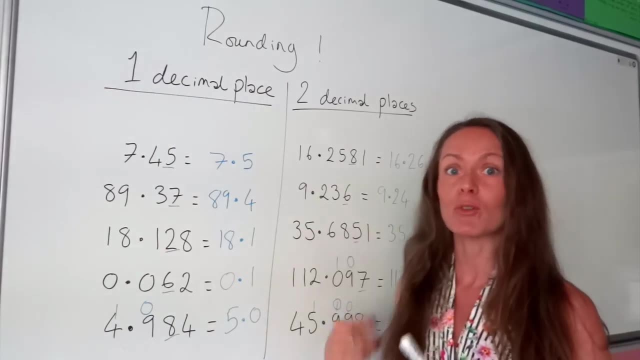 it's exactly the same method. You would just check the fourth number after the decimal point instead, And if you were rounding to five decimal places, you would check the sixth number after the decimal, and so on. But it's exactly the same method. 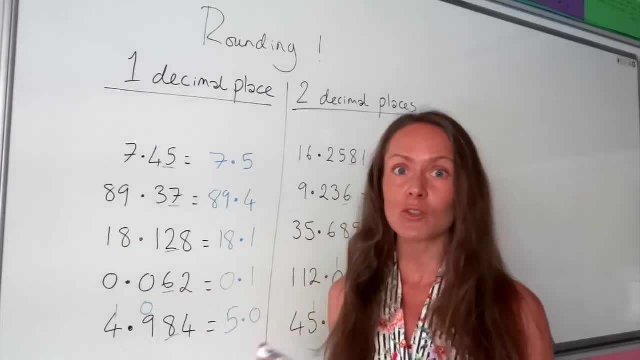 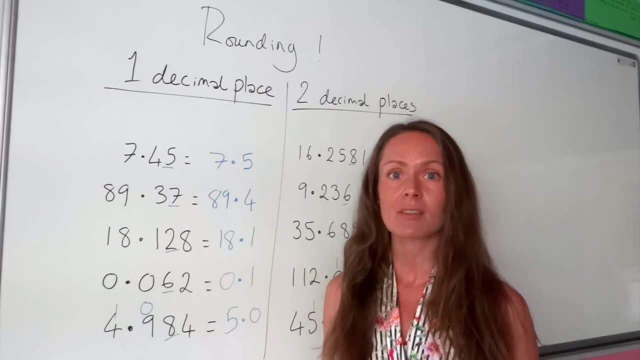 So if you're still a bit shaky on rounding questions, I do have some other videos I've got rounding to three significant figures, rounding to the nearest: 10,, 100, and 1,000.. So have a look at those. 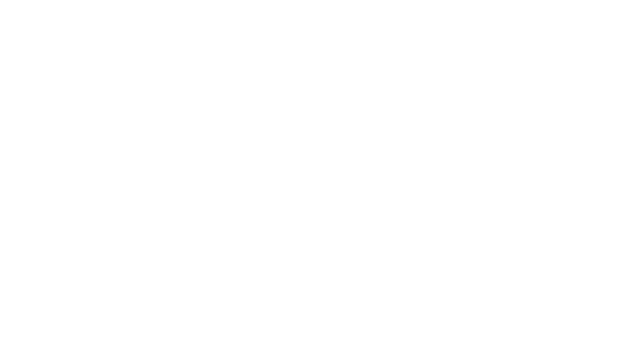 So that's all for today and goodbye from me. I'll see you in the next video, Bye-bye.